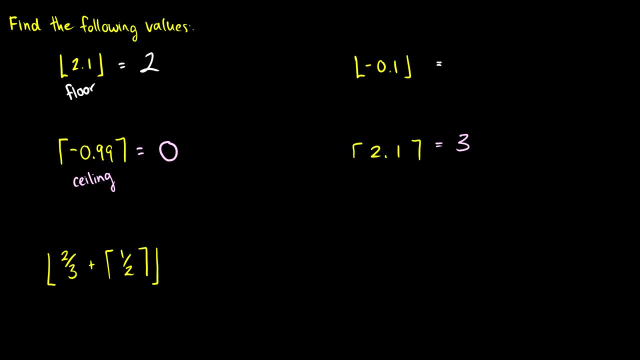 is going to take negative 0.1, round it down so that will end up at negative one. So remember, on a number line, if we have zero here, negative one here. if we put negative 0.1 on the line, it'll be about here. So we round down to negative one. I know it seems like hey, maybe. rounding this down is going to be a little bit easier, but it's not. So we round down to negative one. I know it seems like, hey, maybe rounding this down is going to be a little bit easier, but it's not. So we round down to negative one. I know it seems like, hey, maybe rounding this down. 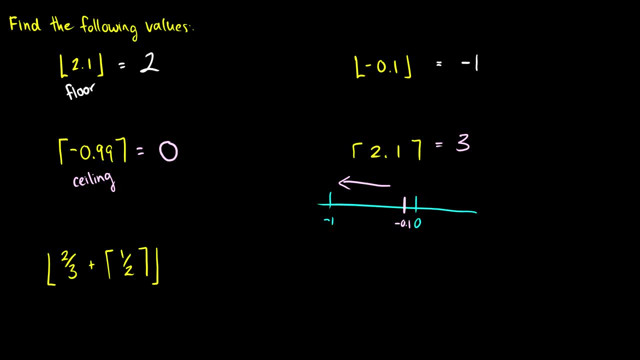 means back to zero. But if we look on the number line and we place these down, if it's the floor, we move left, if it's the ceiling, we move right. So that's how we look at this with a number line. Okay, so let's do a computation question here with a floor and a 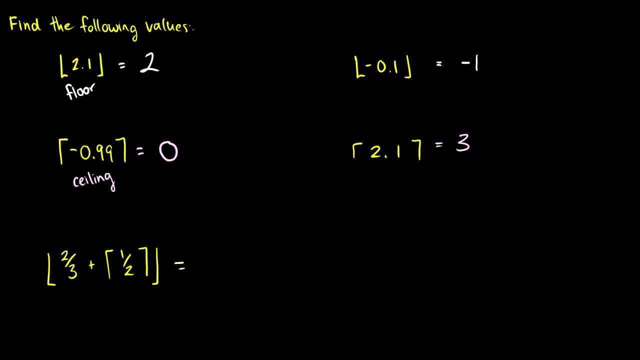 ceiling. So we want the floor of two-thirds plus the ceiling of a half. Okay, so first we're going to do the ceiling of one-half, So we're going to end up with the floor of two-thirds plus the ceiling of one-half. 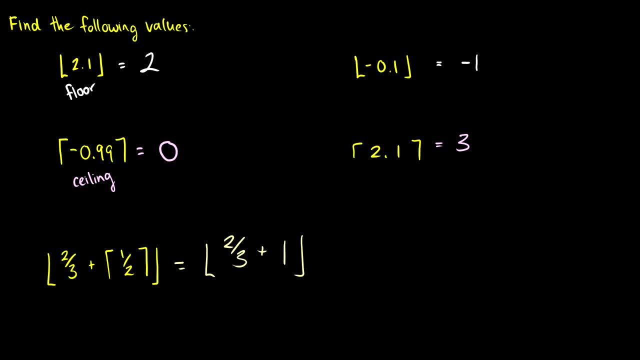 is going to be one. So now we want the floor of two-thirds plus one. So this is just the floor of 1.6 roughly, and that is just one. Okay, so that's some computation questions. Let's give you a formal definition of floor and ceiling. So if the floor 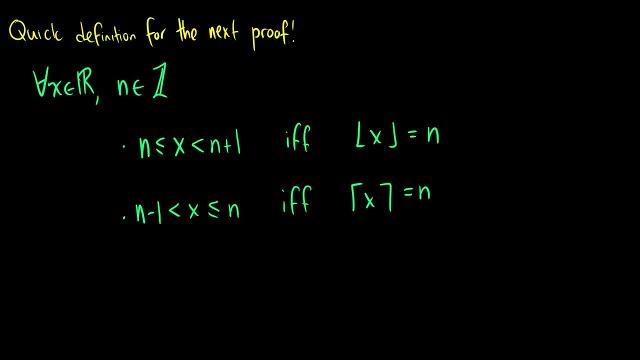 of x is equal to an integer n. so this x is going to be a real number, n is going to be an integer. then we say that x is greater or equal to n, but strictly less than n plus one. Because if x was, 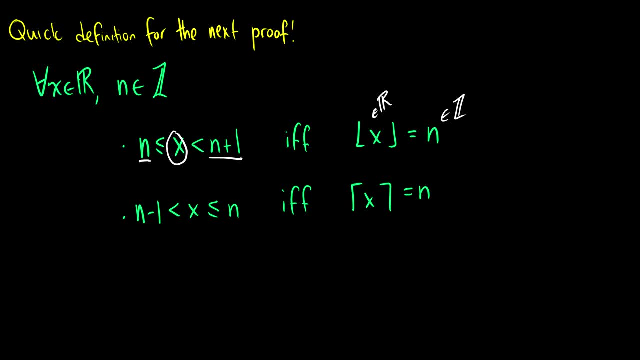 equal to n plus one, then the floor would equal n plus one, So we want it to be strictly less For the ceiling. it's pretty much the same definition. What we're saying here is that if the ceiling of x is equal to n, then x is going to be less than or equal to n, but strictly greater. 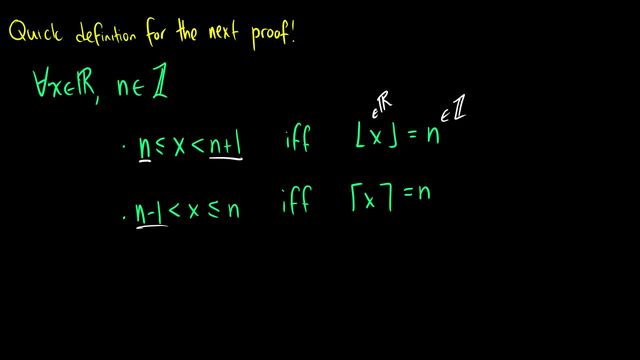 than n minus one. So we're going to use this definition to do a proof here. So what's the proof? Well, for x in the reals, m in the integers, the floor of x plus m is equal to the floor of x plus m. 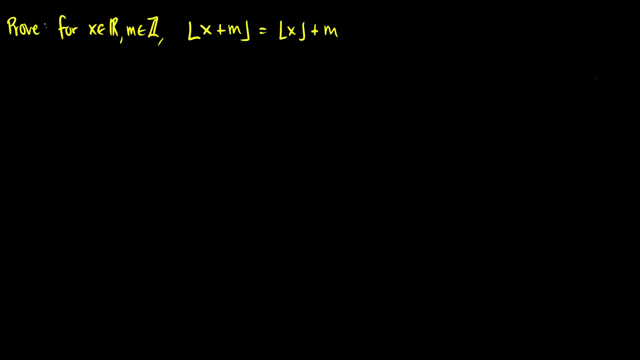 Okay, so what's our definition? Well, if x is, or the floor of x is, equal to n, then x is going to be greater or equal to n, but strictly less than n plus one. Okay, so we want to get the floor of x plus m. 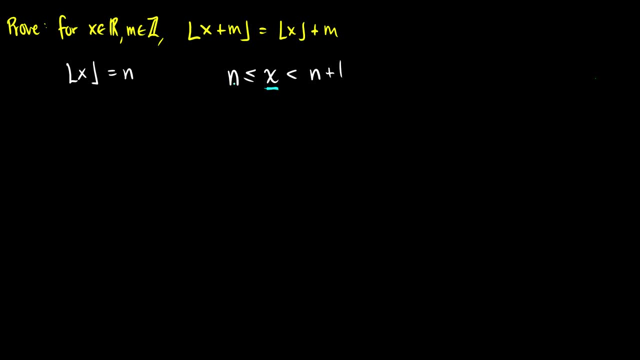 So we already have an x here, so let's just add m into this inequality here. So we're going to get: n plus m is less than, or equal to x plus m, which is strictly less than n plus m plus 1.. So what do we notice here? 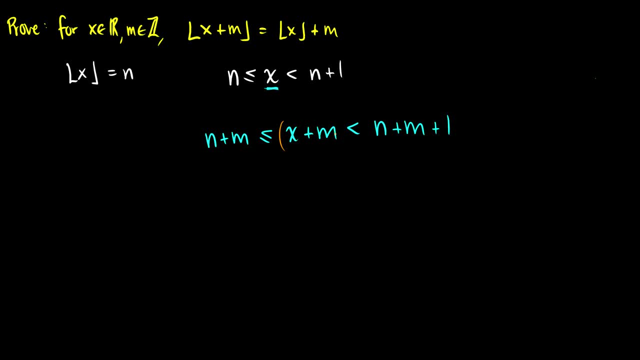 Well, we have the same pattern as our definition. So we can bracket this: x plus m, n plus m, n plus m plus 1, and we see that the definition here. well, if we use the definition, this is like saying that the floor of x plus m 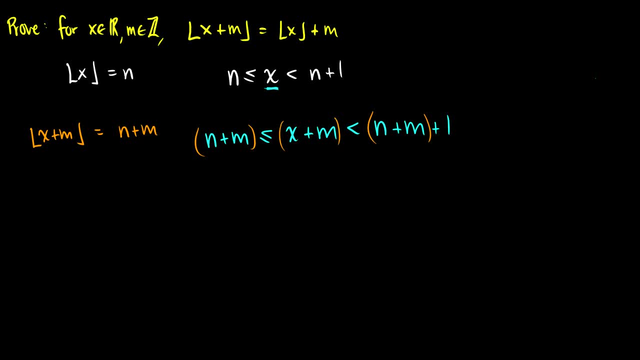 is equal to n plus m. So again, we just added m to each of these statements here, and of course, it preserves the inequality, since all m's are equal. Okay, so now we have this statement: The floor of x plus m is less than or equal to x plus m. 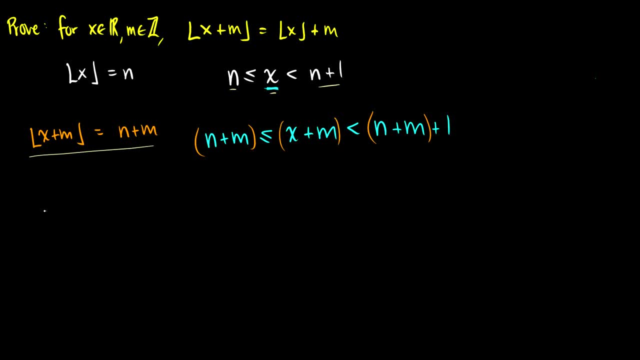 The floor of x plus m is equal to n plus m. but what is n? Well, n we defined as the floor of x. So there we have, a proof that the floor of x plus m is equal to the floor of x plus m. 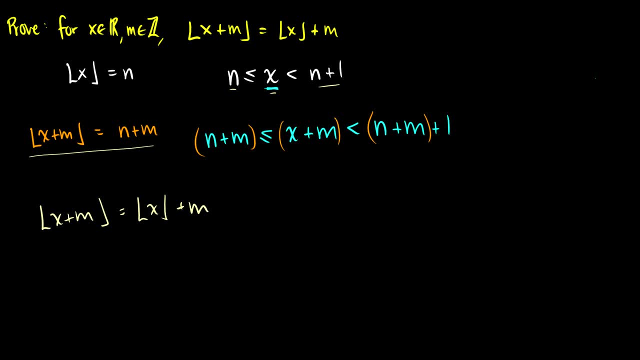 Okay, so that's it for ceiling and floor functions. Of course, what you can do is you can try to do the same proof with ceilings. So check it out, post it in the comments if you have a solution- and, of course, there are many more. 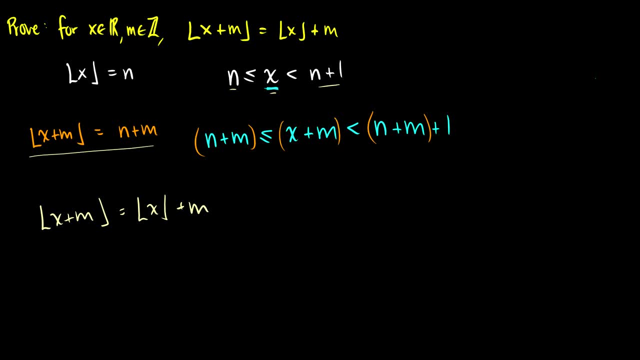 There are many more proofs that you can do as well, so you can check online for those. I may do another video on it, but it's not planned in the near future, So please leave your questions in the comments below and I'll answer them the best that. I can.